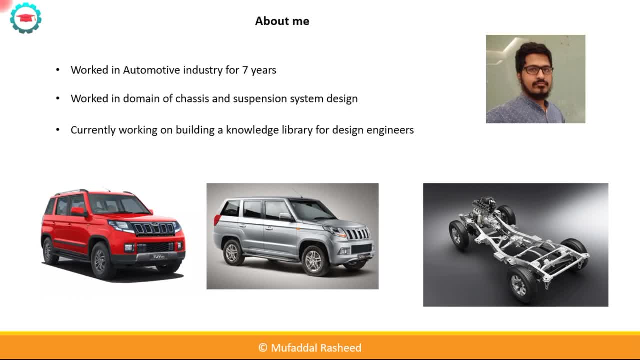 a course. Well, basically, I am a design engineer who has worked in automotive industry for seven years and I have worked primarily in the domain of chassis and suspension system design in automotive product development. I have been part of the vehicle design and development team in SEV projects and I have seen projects from concept to production Through my experience. 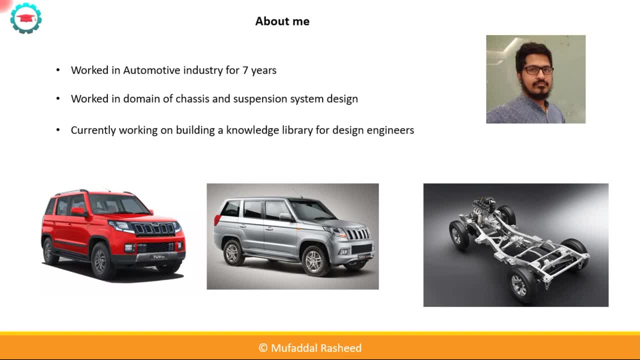 I have developed a deep interest for mechanical design engineering and currently I am working on building a knowledge library for design engineers for the reason for enhancing knowledge and upskilling. So this course is basically an attempt to share whatever knowledge I have gathered as a design engineer and whatever insights I have gathered about the profession, about the 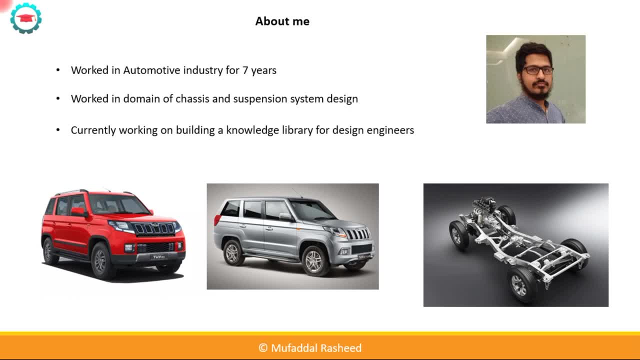 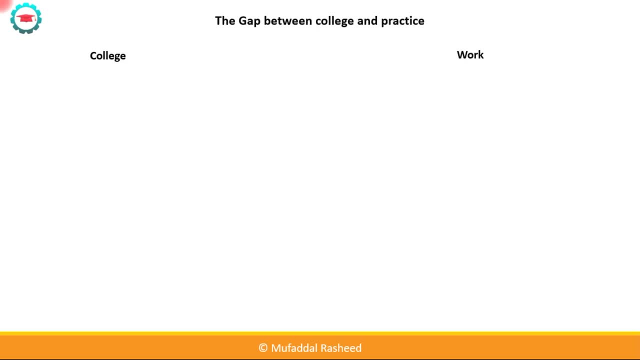 role. So this course is basically my perspective or my world view with respect to the design engineering profession. So we will start by understanding the gap between the college and practice, or when you are actually doing the work, when you are delivering. what is the gap in the skills and knowledge required? So what you learn in college versus what you are required to. 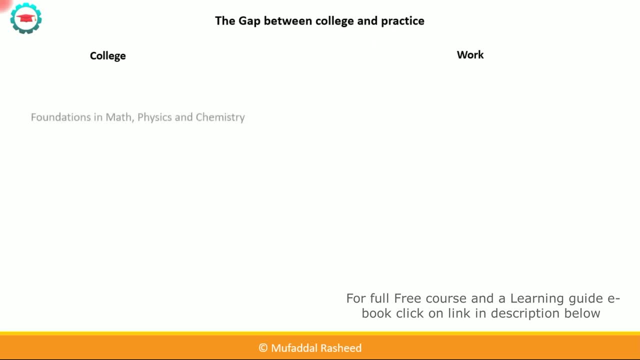 know in work to deliver. So in college we learn about the foundations of math, physics and chemistry. Both school and college we learn all of these stuff and we learn about engineering subjects like strength of materials, mechanics of materials, engineering mechanics, kinematics, dynamics, fluid mechanics, thermodynamics. all of these would be the basics, and 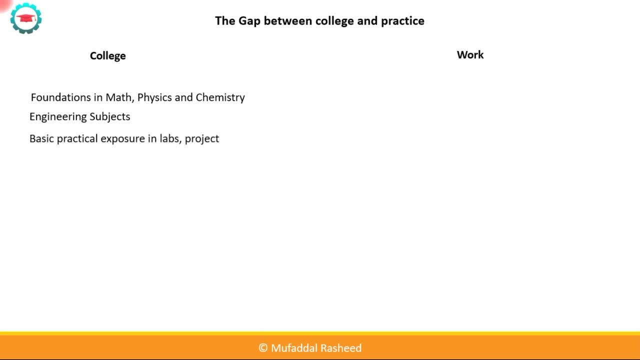 we get some basic exposure in the form of labs and what projects we do. So this basically builds a type of engineering literacy. So this makes us ready for an engineering job. Basically it provides the basic, foundational, fundamental information or fundamental mindset to become an engineer. 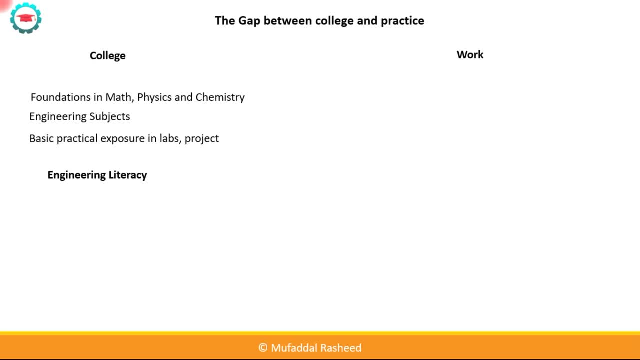 But engineering literacy alone cannot give us products. So the idea of most businesses in the product development or manufacturing space is to develop products which solve problems for society and they gain profit out of it. So that motive is satisfied by converting engineering literacy into engineering practice. 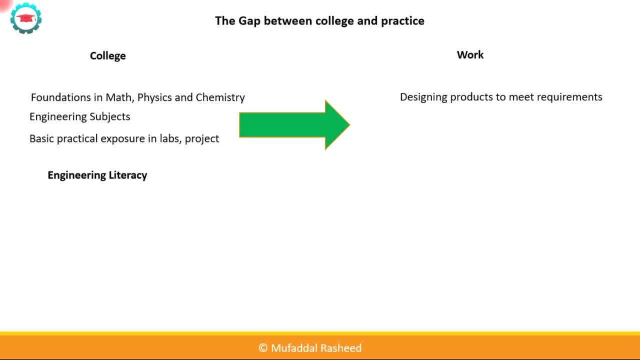 So this has to be converted into skills which allow a person to design products to meet certain requirements, to solve practical issues in products so that they can be resolved, and to make designs manufacturing. So these kind of skills are required for business and this is called as the engineering practice. 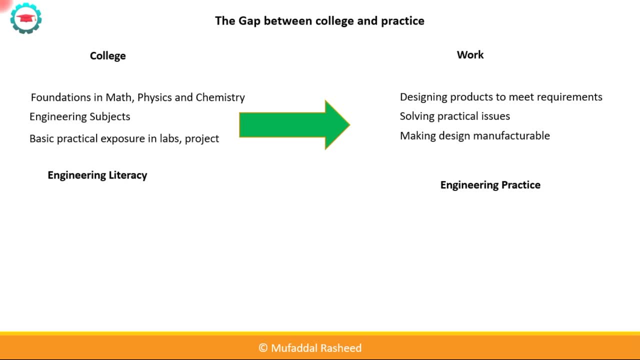 So, basically, when you graduate and when you start working, you apply whatever you have learned during the college studies, which is engineering literacy, into practice to design products. So if you want to transition from being engineering literate to being an engineering practitioner who can design products for business or for societal impact, 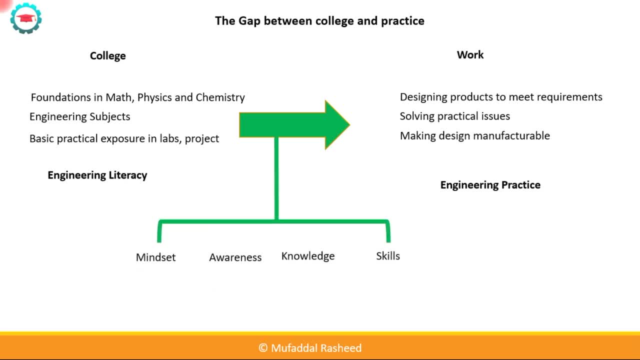 Then you need a certain level of mindset, awareness, knowledge and skills. Of course, this is considering that college does not teach you these skills outright. To share with you my experience when I graduated out of college and started working, I learnt a lot in the first year about how product development works, how the basics of engineering which we 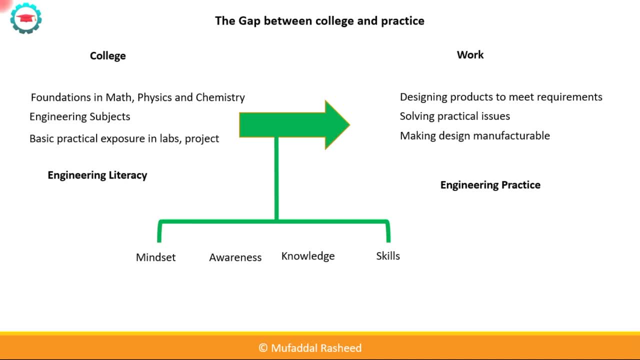 learn in college are applied to design products, and also I learnt about many new skills which are which how to be developed and which are applied while doing the projects, and skills which are developed primarily through hands-on experience, while working in the project and being in the thick of it. Now we will understand the big picture: the impact of a design engineer in a 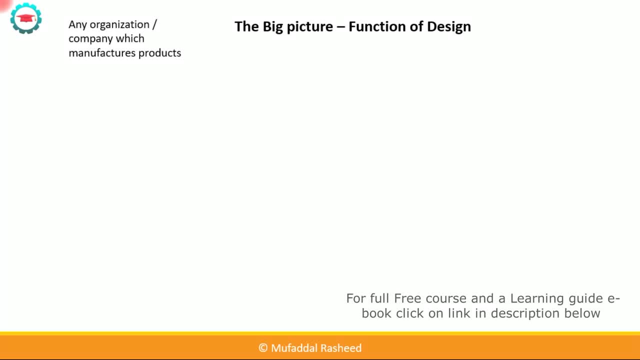 manufacturing company. So any organization, company which manufactures products will have three major functions or three major departments, that is, design, manufacturing, marketing and sales. So these three functions make up the whole product development. So the product development, the conversion of a product from idea to something which can be. 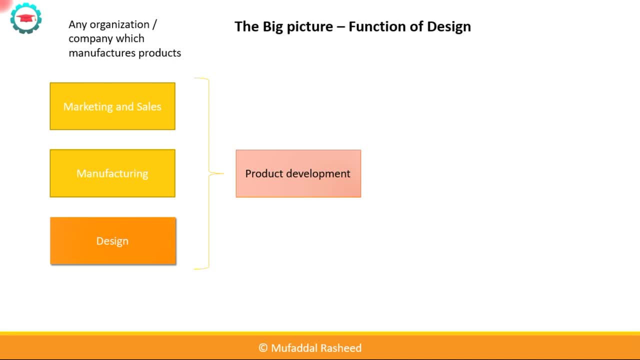 monotized and sold in a market, requires three functions: design, manufacturing and sales, And that in turn generates the business, generates the impact or the wealth. Now, over here, design is where the product is conceptualized and created. So if we go into the 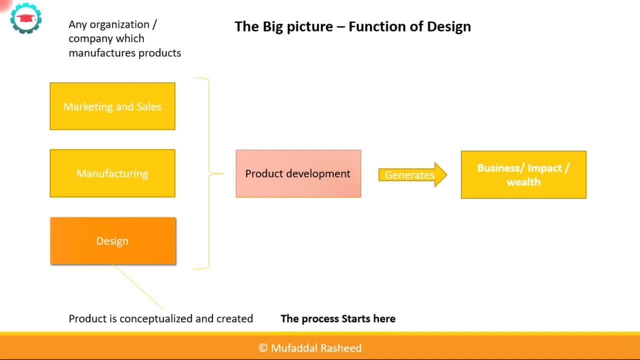 So it all starts from here. The product development process starts from design and ends at sales. Hence you can make out the impact which a design engineer has on the final business of a company. If the design is good, there will be good sales. 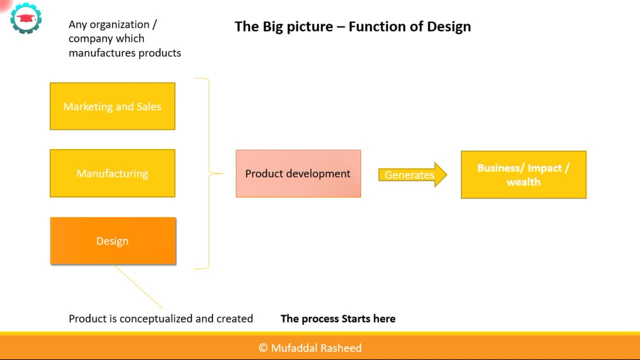 If the design is bad, then the sales will be affected. So the design directly impacts the business of the company. So, apart from creating designs, design engineers also improve the designs So they can optimize the cost of the designs. Let's take a simple example. 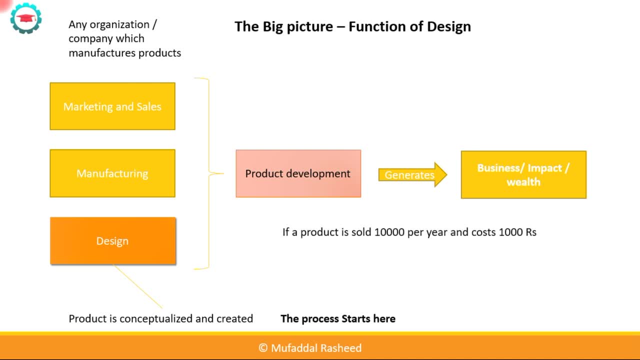 If a product is sold 10,000 times per year, that is, the volume is 10,000 and it costs 1000 rupees. If the design engineer optimizes the design and reduces the cost by rupees 50,, then the 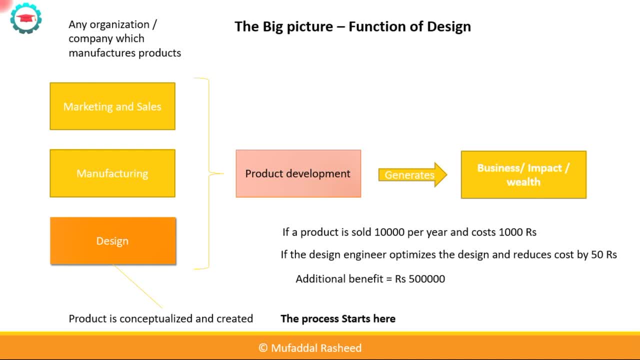 additional benefit for the company is rupees 5 lakhs or 500,000.. This is considering the fact that no changes have been done on the manufacturing process. Similarly, any small changes in the design can have massive impact on the business. 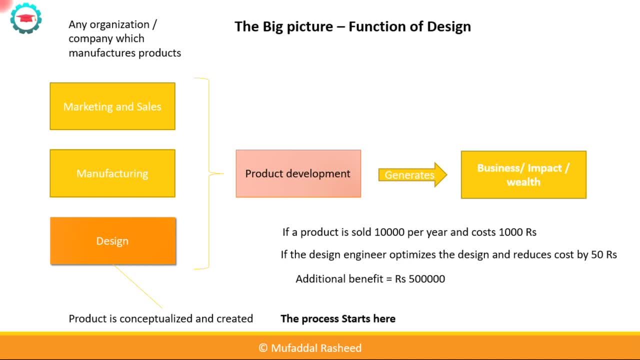 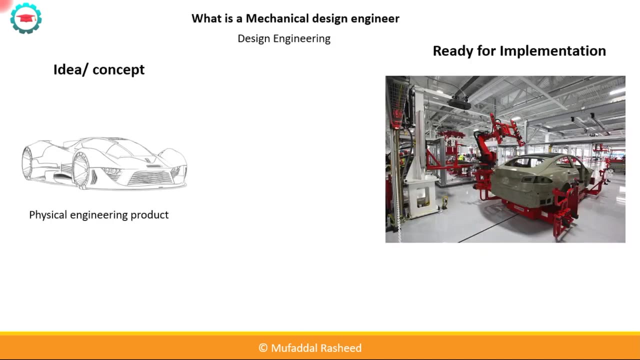 It can be highly positive or, in the other hand, it can be highly negative also if it is not done correctly. So this is the impact of a design engineer or a designer in the overall product development in a manufacturing company. Now let's have a look at what exactly is mechanical design engineering in the context of product. 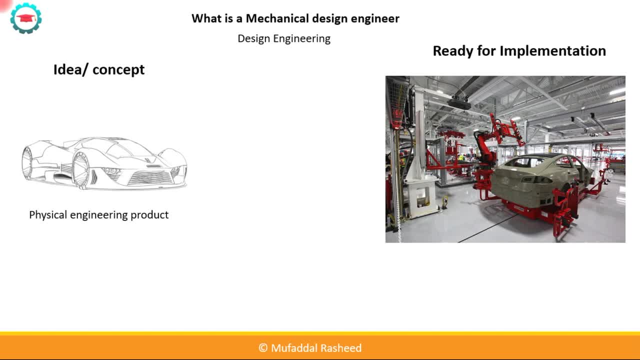 development. Now let's say we have an idea or a concept of a car Which is basically a physical engineering product, and we want to take that idea or concept from sketch or from the 3D model into something which can be made ready for implementation. 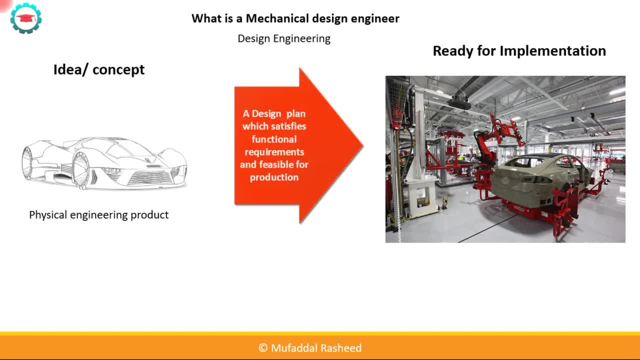 ready for production, So that transformation of an idea or concept into a design plan which satisfies certain functional requirements set out for the product and is feasible for production. this transformation from the idea level or concept Level to the ready for implementation level is called as the mechanical design engineering. 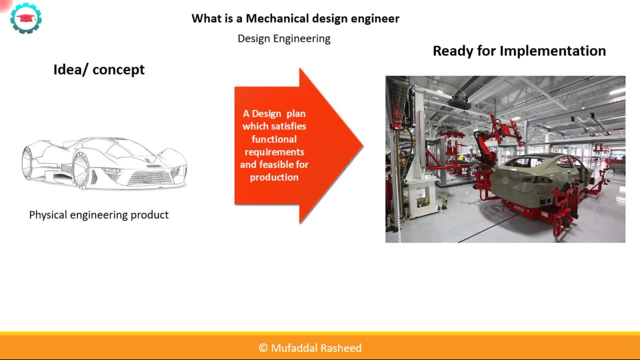 This is specifically for a physical engineering product. So this design plan will generally consist of a lot of design documentation, which will include drawings, which will include a set of instructions on how to assemble parts, which would also include the analysis reports or whatever analysis or validation has been done. 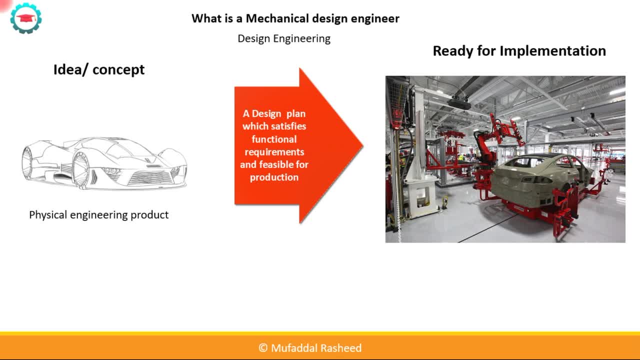 on the designs to prove out their function. So all of that combined will make the product suitable for production and such that it can be sold in the market. So this requires three major activities. One is to create the design, that is, conceptualization. creating the package, creating the base level. 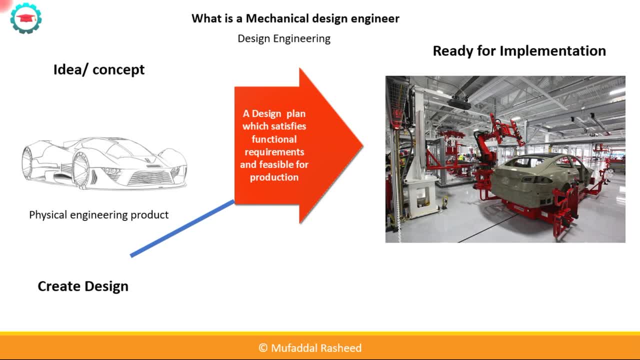 mechanisms, structures which are required, like, for example, the body structure, the shell structure has to be designed, the chassis structures has to be designed, the various mounting schemes how to be designed. So all of that comes in The create, the design. Then we have analysis and testing. 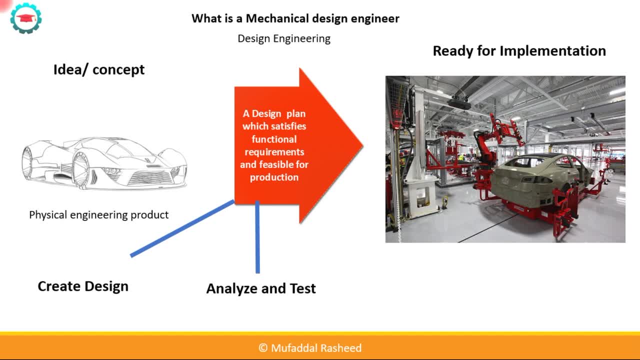 So, whatever designs are being done, how to be analyzed, how do we evaluate it based on its functional requirements, whether it be durability or safety, or reliability and various other aspects, for example strength. when we are designing a bracket, we need to test it for strength and then making it feasible for production. 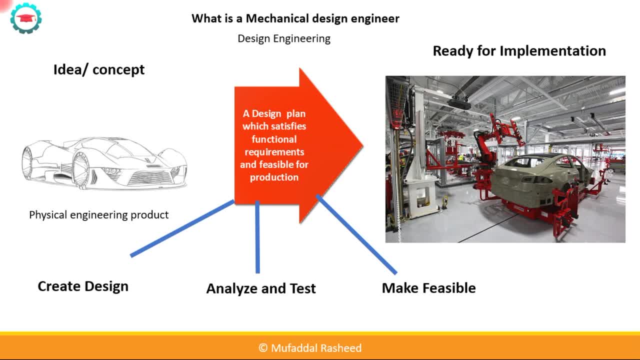 So whatever designs we make Are not readily manufacturable. we need to make them manufacturable such that they match with the production processes or manufacturing processes which are available. So this is a simplified overview of the task of a quintessential mechanical design engineer, which is to convert an idea or a concept into a design plan which is ready for implementation. 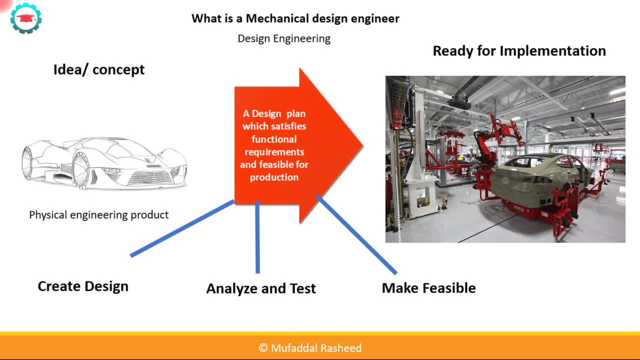 or ready for production. For doing this task of converting a concept into a design plan which is ready for production cannot be done by a single person, Especially for a product which is as complex as a car or a vehicle or aeroplane or any of that sort of a product, which is basically a system of systems. 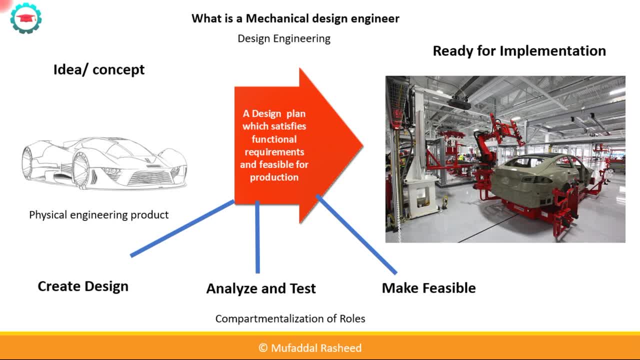 In that case compartmentalization of roles and the role of system engineering comes into play. So, basically, you divide the whole product into various systems and there are various teams allotted to them and they work on various systems, Systems like the power train, the body, the chassis, the suspension, the wheels, etc. 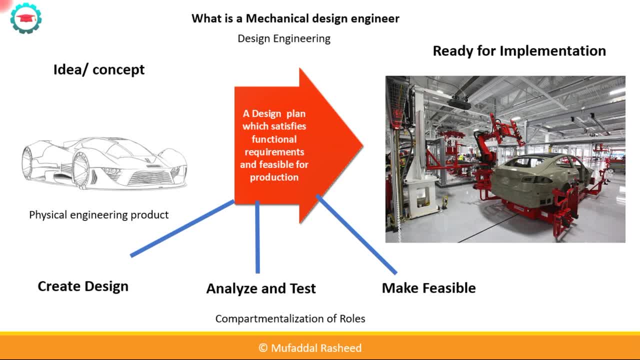 All of those system teams are divided and there are people working on different aspects, like some design, some only do analysis, some only do the testing. So that way this compartmentalization of the larger role of design engineering is done in the organization which manufactures cars or it manufactures very complex products. 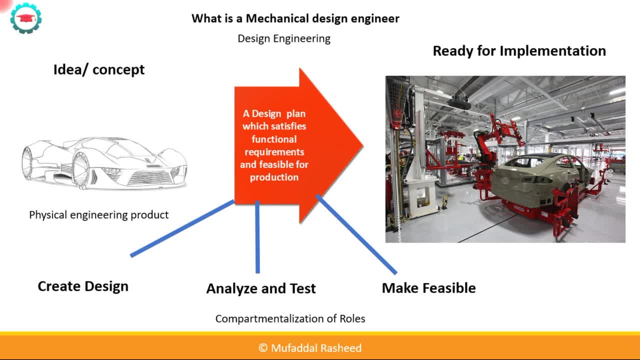 But in the case of simpler products, products which are having lesser number of parts and lesser complexity, This whole process of creating a design, Compartmentalizing and testing it and making it feasible for production can be done even by a single person, if he or she has that required knowledge and skill sets. 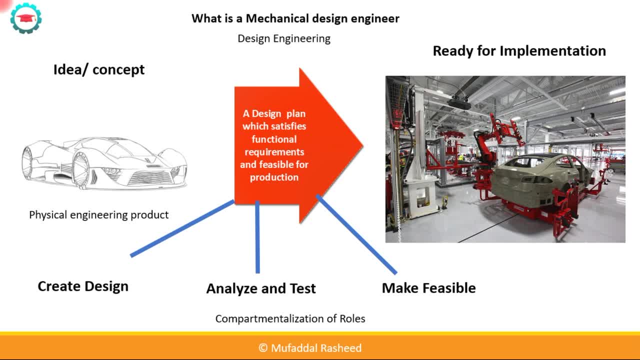 So it is important to note that with compartmentalization of roles, the skills and knowledge required in specific roles becomes highly specialized. Hence, if you are working in analysis, you will only be doing analysis. you will not be creating concepts or creating designs or making designs manufacturable. 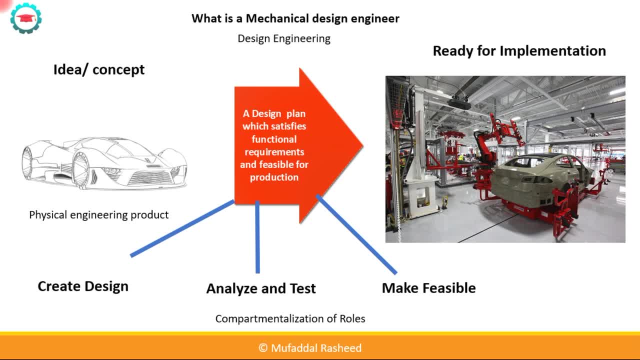 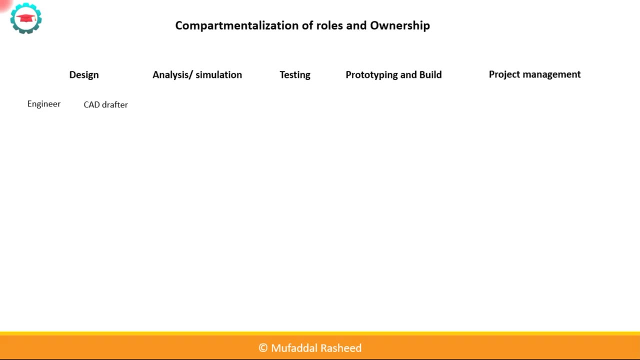 So you become highly specialized in that area. On the other hand, if you are working in testing or validation, you will be highly specialized in the validation and testing of various components, whether it is in the lab or whether it is in the real world. So the compartmentalization of roles in the case of vehicle product development or product 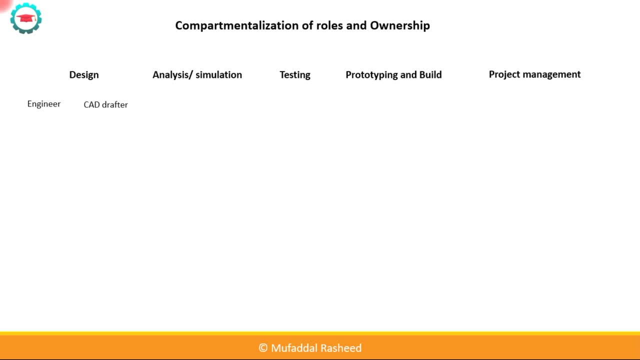 development of systems will be something like this: there will be a central design team who will have the ownership of the design, Who will create the designs and then give out the designs for analysis, for testing, for prototyping, and also coordinate with those teams to make the design ready for production. 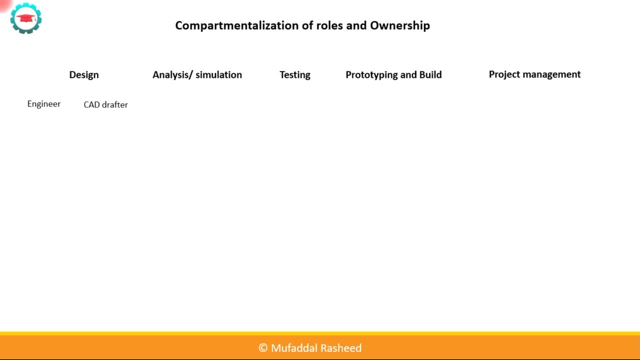 And then there is the analysis or simulation teams who will do analysis, like strength analysis, durability analysis, vibration analysis, fluid flow analysis, thermal analysis, and they are specialists in those areas. Then there is a testing team who takes the design Or takes the manufacture or prototype from the prototyping teams and tests the prototypes. 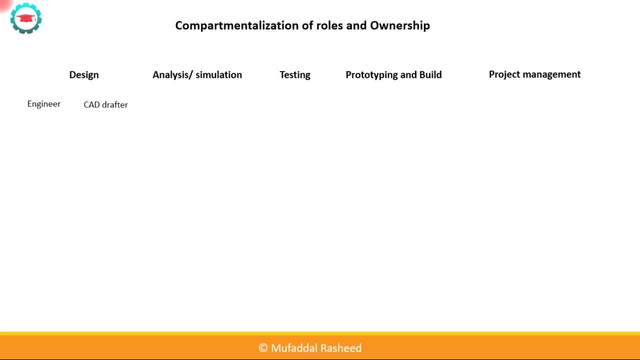 such that they match the requirements which are set forth by the design engineers And then the prototyping and build team. they take the designs from the design engineer and make the prototypes as per their requirements or as per the milestone of the products, And then project management will handle all of the other administrative activities which 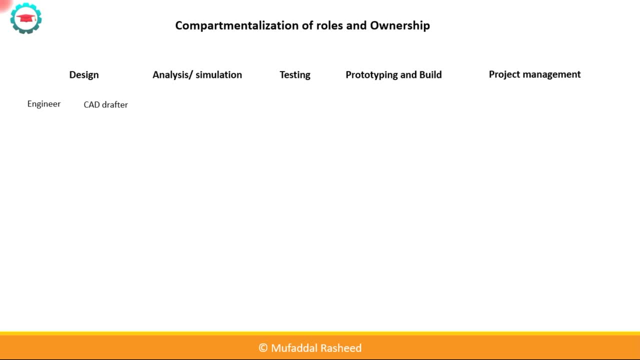 are required for making sure, Making sure that the design, That the design is done project goes in a smooth manner. so under design role there can be an engineer and also a cad designer or a cad drafter. so the job of a cad designer or drafter is to just make cad models. 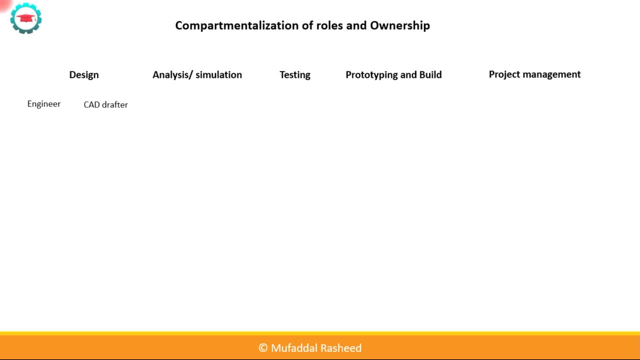 and drawings on the directions of the engineer. so this is a way in which the compartmentalization of roles happens. now, of course, we are dealing with design engineering over here, so we are going to talk primarily about the design role. so the original work which we had seen in the earlier 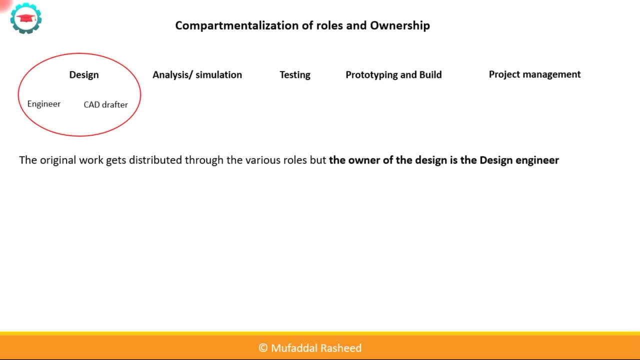 slide has got distributed to various functions, but the final ownership lies with the design engineer and whatever decisions are made, the design decisions which are made have to be made by the design engineer with respect to various aspects, whether it is the aspect of durability, or whether it is the aspect of functionality, or whether it is the aspect of 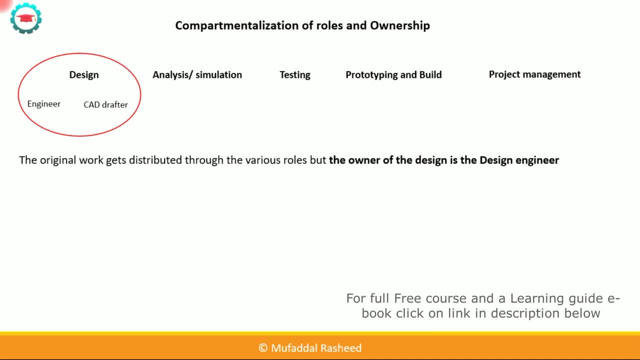 feasibility for manufacturing. design engineer is the final decision making authority for the design. so in a way, we can say that the designer design engineer is the creator as well as the decision maker for the design in the product development, whereas the other roles, like analysis, testing, prototyping, are assisting the design engineer to make sure that the design comes out. 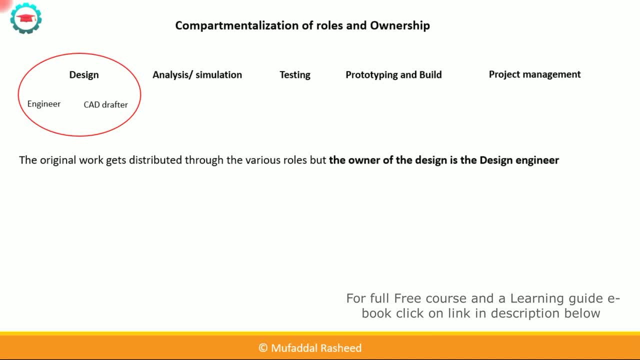 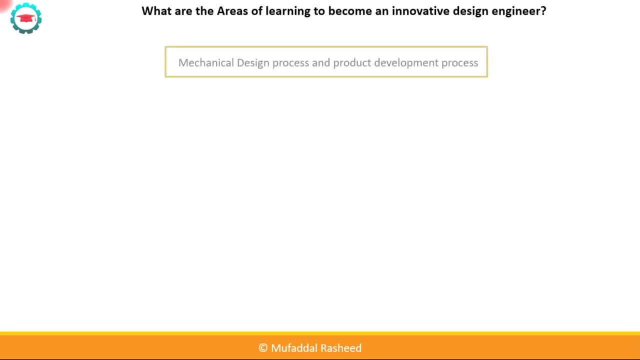 to be high quality and highly efficient and optimized. now i will summarize: what are the roles of design engineers, as in design engineers? are the design engineers, are the designers of design? What are the areas of learning to become an innovative design engineer? So the first thing is, and the most important thing is, understanding the process, that is. 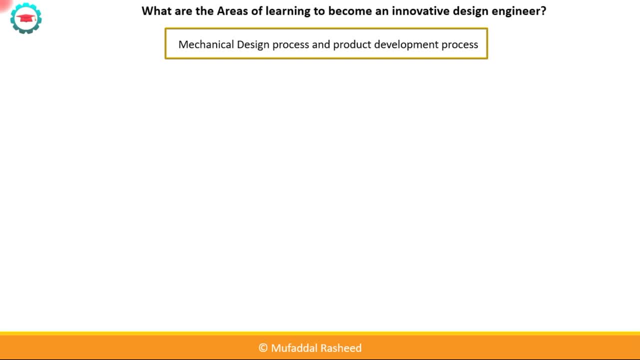 mechanical design process or product development process. When you understand the process, you can organize your effort in a much more efficient manner. This is a very important thing to learn when you're in the practice, because what happens is when you come up with an idea, you develop concepts, you develop the designs. 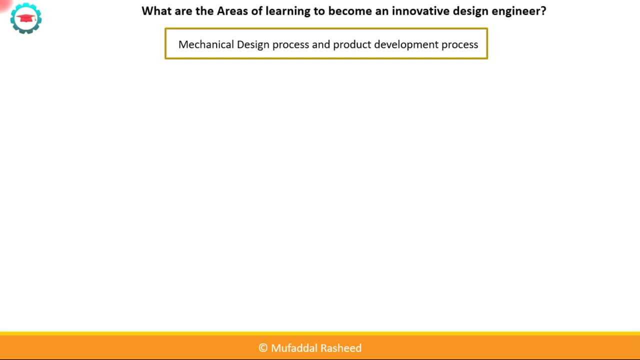 It generally happens in a haphazard manner and not in an organized manner. Having an organization and doing it in a very methodical way is very important to get good results. So the first thing is to understand mechanical design process and to understand the overall 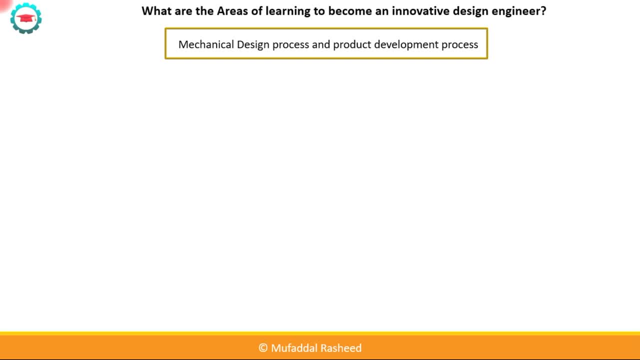 product development process of various products. This knowledge is also helpful in terms of the job growth, because when you are understanding the process, the way people work in an organization, You have very high chances Of growing to the next level because you understand how things takes place, how product 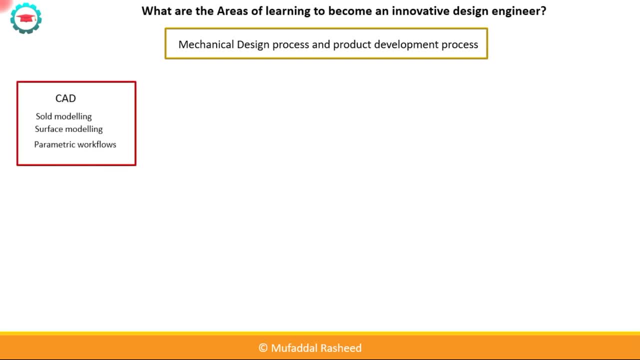 development takes place. The next is obvious one, which is CAD. So design engineers should have very good hold on solid modeling and surface modeling and should be able to come up with parametric workflows which are editable, which are modular and which can be modified easily later. 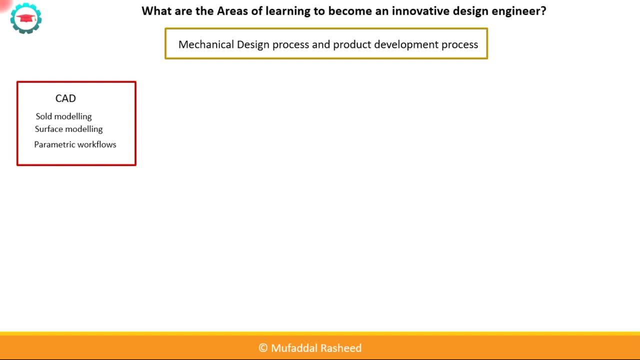 So developing CAD skills is a very important part of the skill set. CAD skills can be developed By working on various types of projects and basically understanding the different types of workflows for making different types of geometry. So that is all based on practice. Next important area of study is engineering drawing: GD&T, tolerancing and fits. 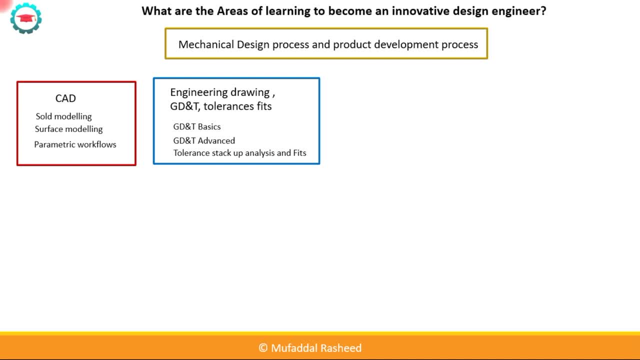 So, basically, in any organization which is manufacturing products, there is a stage at which the designer has to convert the designs into engineering drawings, And those engineering drawings are basically the documents, The official documents, The documents of the parts or components which the designer is designing. 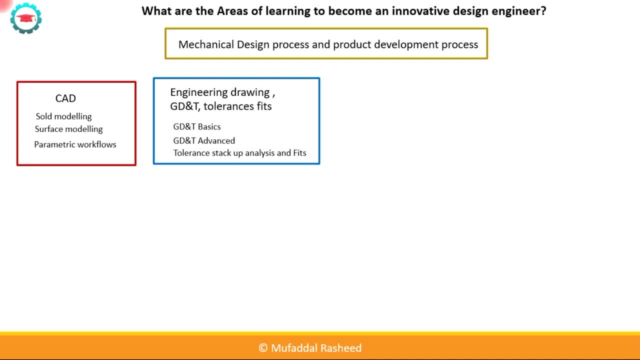 And that will be the reference for the manufacturer and the inspector. So preparation of engineering drawing is a very important skill and very important knowledge, or knowledge set for a design engineer. And during the course of preparing engineering drawings we apply GD&T geometric dimensioning. 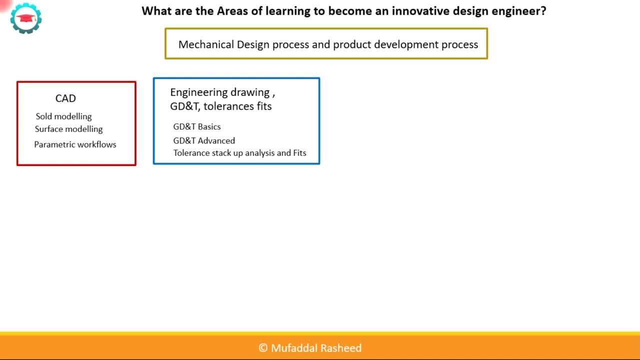 and tolerancing And that is a tool set which is used for conveying design intent. It is a very important skill set And related to that is the understanding of tolerance stackup and how to analyze the tolerance stackups in an assembly. Also the types of fits which are there and how to interpret them and how to specify the. 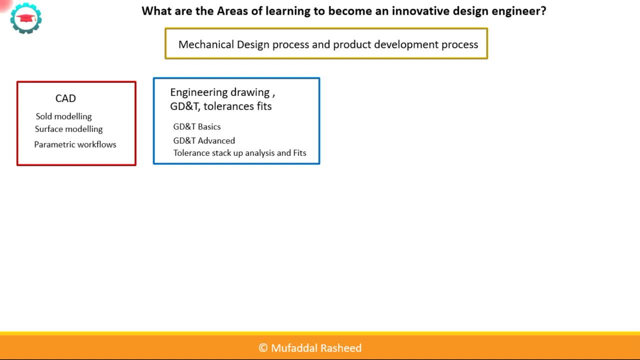 fits. That is a very important skill set while preparing the engineering drawing. Next area of learning is basically the application of engineering basics or engineering concepts, Concepts like mechanics, machine design, engineering analysis. So subjects like mechanics of materials, statics, dynamics. 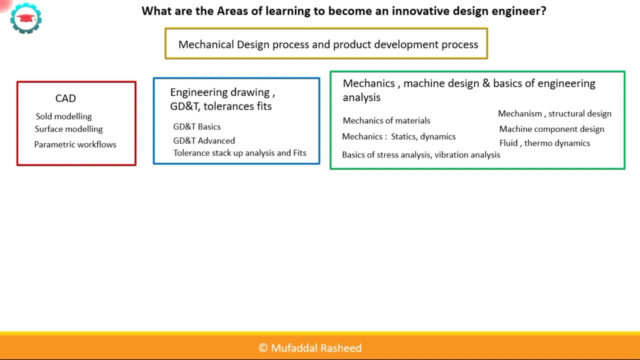 Mechanics of materials, Mechanics of materials, Mechanism and structural design, machine component design, fluid mechanics, thermodynamics, stress analysis, vibration analysis- all of those would come in this area of learning. Next is understanding of materials and manufacturing processes. So material properties. understanding material properties is a very important knowledge set. 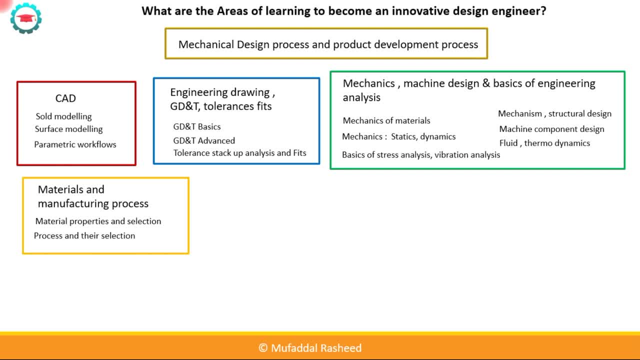 for design engineers, because when you understand materials properly, you can utilize them in the most efficient way in a design and hence you can select the most optimal materials for the application. Similarly for the manufacturing process, And when you understand manufacturing processes, you understand the parameters which are going. 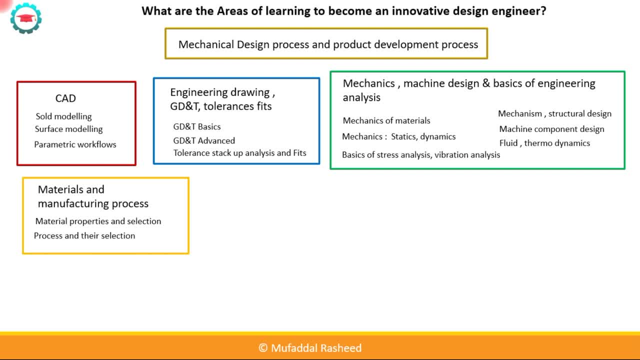 into play to decide the dimensions of the part. So that is a good amount of relationship between manufacturing process, materials and the dimensioning and tolerancing of the parts. So a good theoretical as well as practical understanding of materials and manufacturing process is a very important skill and knowledge set for design engineers. 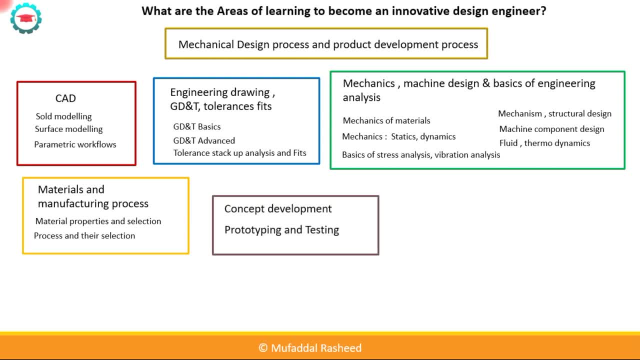 So that has to be developed. Next area of learning is concept development and prototyping and testing. So concept development is basically the phase in which you are ideating, you are developing ideas, you are developing concepts, you are sketching the concepts or you are making rough. 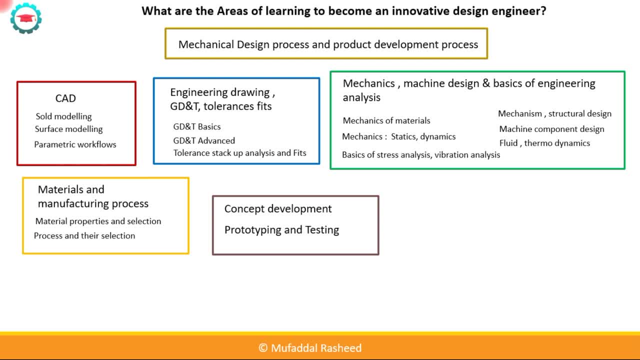 CAD models of concepts. you are just trying out different things. So it is highly creative phase And this is the area where the creative problem solving part has to be developed. So the skill of concept development has a lot to do with the creative problem solving. 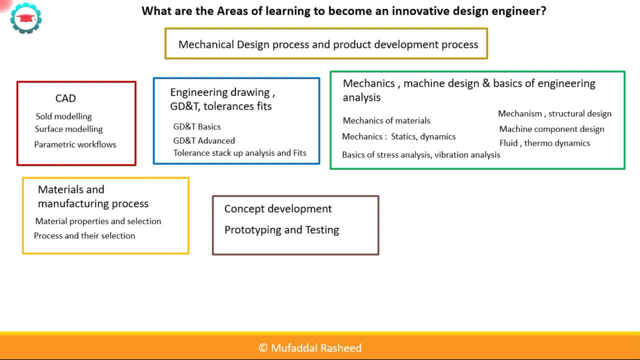 skills. So if you are highly creative and if you are having good amount of background knowledge, you can develop many different types of concepts. One important thing to note over here is the quality of concepts you generate depends on the background knowledge you have of the other domains. 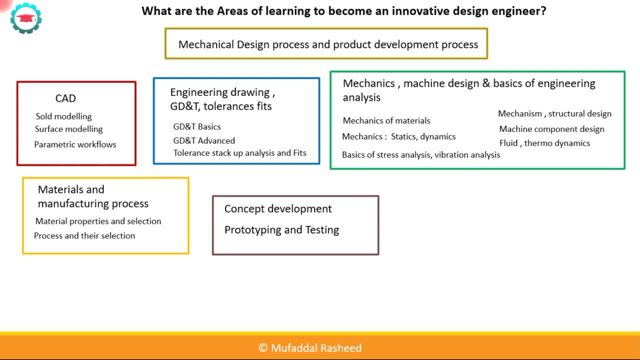 Like, for example, if you have some knowledge about different types of structural concepts, if you have knowledge about different types of concepts of mechanisms. let's say you know about 10 or 15 different types of mechanisms, like a four bar mechanism or a slider crank. 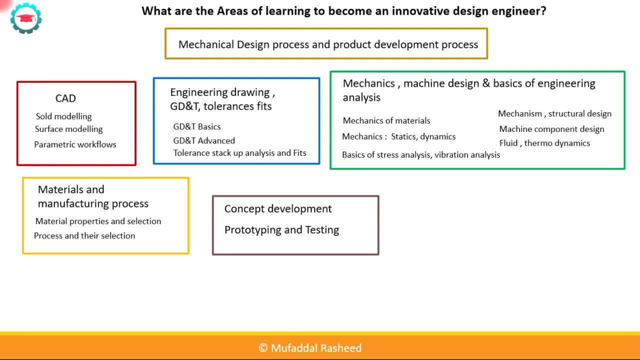 mechanism. whatever those background knowledge is, those things will actually guide your concept development thought process. So of course it is subconsciously done. it is not done actively, but as and when you keep on gaining knowledge, your concept development skills will also keep getting better. 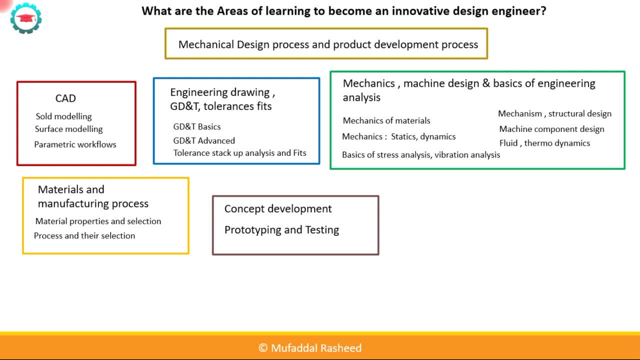 And they will keep getting better as you work on more challenging problems. So the more challenging the problem is, the more you will have to think about developing the concepts. And the next skill is prototyping and testing, Which is basically the usage of different types of manufacturing processes, or you can. 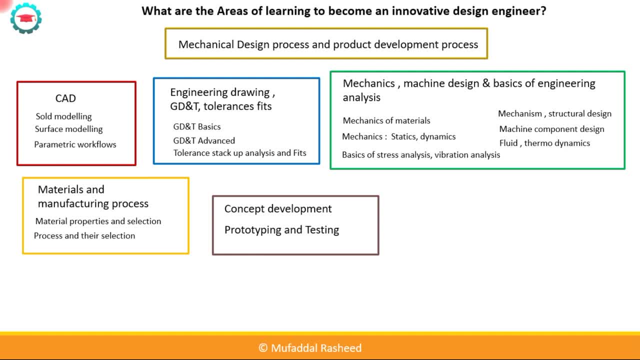 say, cheap manufacturing processes which can be used for making prototypes, which are temporary and only used for testing some aspects of design or testing some functionalities of the design. So the strategy you employ in making prototypes and the choices you make for materials and the manufacturing processes, all of that is generally developed with practice. 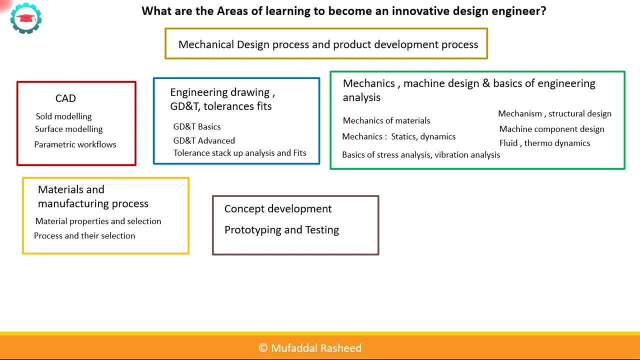 And with regards to testing, testing, experimenting and observation is a big part of learning for a design engineer, especially when you're doing new types of design. So, when you're doing new types of design, you do not have any legacy data or legacy information. 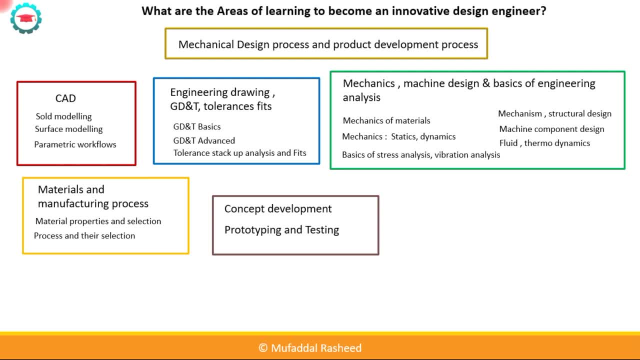 You have to devise the experiments or testing to actually extract the data, and extract meaningful data which can be used for the validation of the design. So that in itself is a separate skill. And then we have design for manufacturing and assembly and design for X Where X can be. 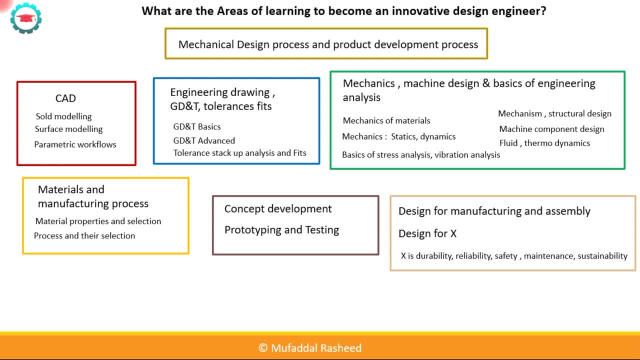 durability, reliability, safety, maintenance, sustainability, which is basically any product requirement depending on the application. So generally, it is the aim of the design engineer to design products which are easy to manufacture, easy to assemble and which are low in terms of manufacturing cost. 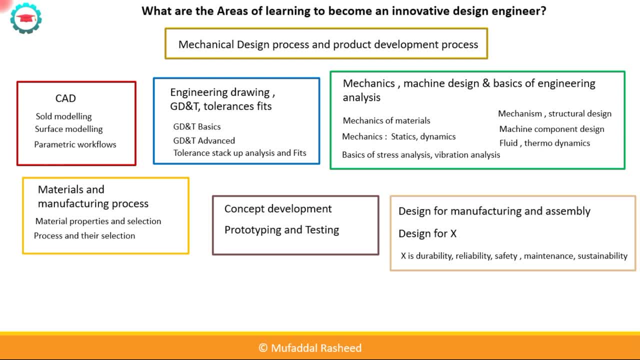 So design for manufacturing and assembly becomes a crucial activity for the design engineer. Developing this skill or developing this knowledge set, is purely based on practical experience and working on various types of projects which have to go for manufacturing, and you have to optimize the designs for the manufacturing and assembly. 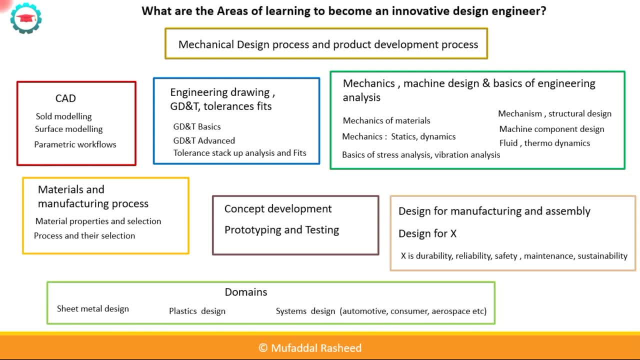 And then we have domains. So domains are basically certain areas of specialization like sheet metal design, plastics design. Those are their own specific skill sets and specific knowledge sets. And then there are systems design, which is basically related to the various different types of systems, specific to the systems: automotive systems, aerospace or consumer. 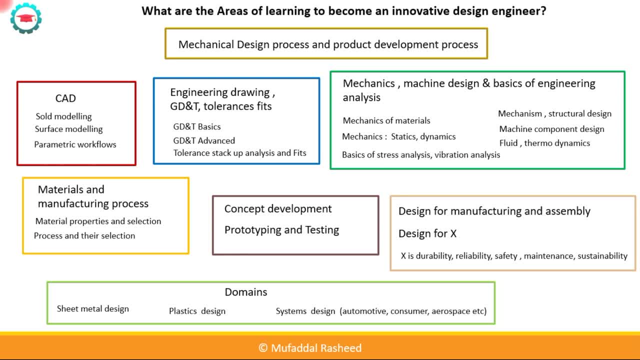 products or industrial machinery or construction systems, whatever the systems are there. based on that, you have to design. So this is basically specialization of the design engineering. So all of these on top, before the domains, are all generic skill sets or generic knowledge sets for design engineers which have to be developed, and the domains signify these specializations.